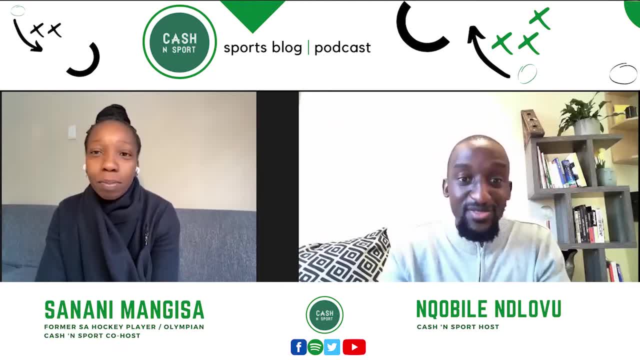 olympics, uh, but no fans, yeah, no fans of the opening ceremony, but the vips allowed, which is an interesting one, um it. you know it goes to who's really who are the olympics for, but uh, yeah, that's, that's been an interesting move for the ioc. yeah, and the nice one is, yeah, nursing moms are allowed. 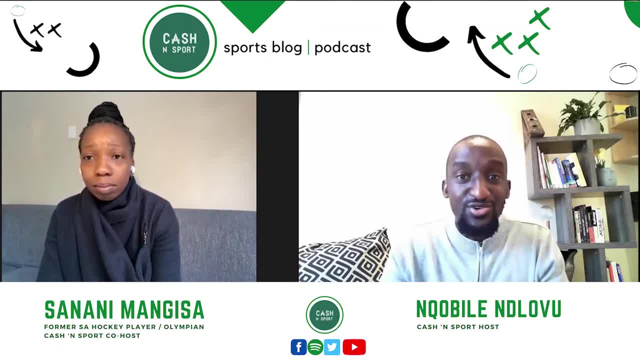 as well, um to uh to bring their children to tokyo, um, yeah, but there's also been mudslides in japan, you know, and there's been covert breaking out everywhere, you know. i mean with with the south african teams, um, with the british and irish lions tour now up in, up in smoke. yeah, we don't know what's gonna. 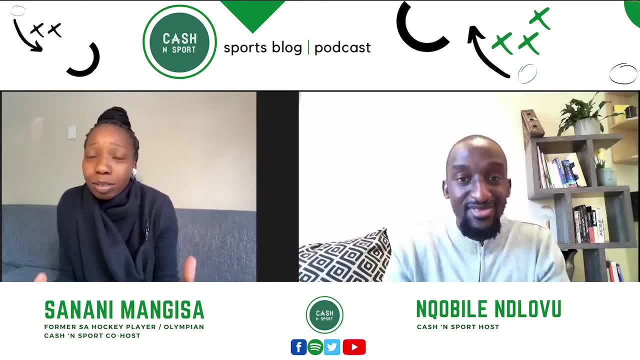 happen. i'm sure the isc are looking at this going: oh, you know, this is this. this is on a small scale and then the eye and the limp is on a bigger scale, more extrapolated. so i can imagine someone is watching this at the isc going: that's not, that's not good for us. but you know, and and also just to 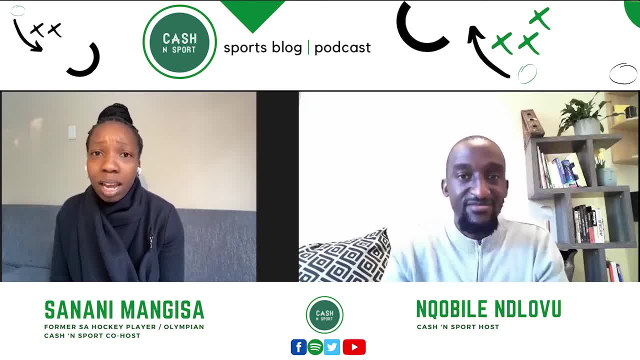 put it out there: all the boxes are vaccinated, and the local teams, so vaccination is not an issue. everyone's vaccinated. it's just that coverage does spread even if you are vaccinated. um, that's what we're talking about today, 16 days away from the start of the olympics, and um, we are. 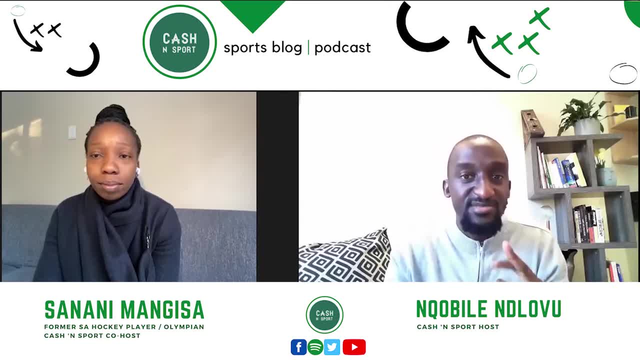 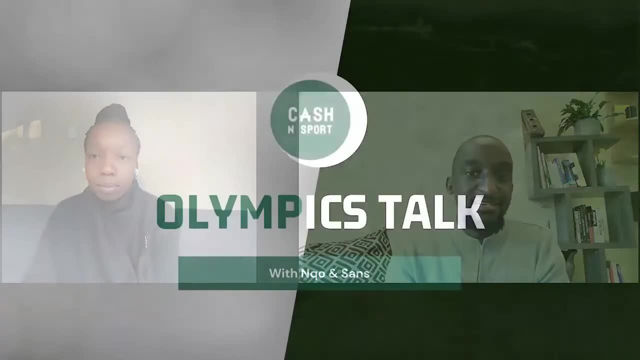 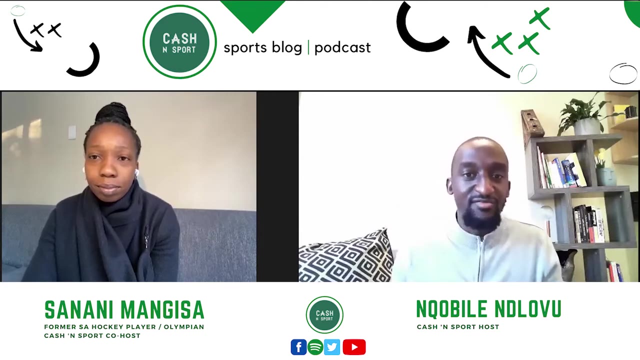 mainly looking at the money around the olympics sponsors, um, how the ioc is funded, what they use that money for. you know, broad cost revenue and just the general money side around this big behemoth that is the olympics and um. to start it off with um, let's take a look at the, the funding. 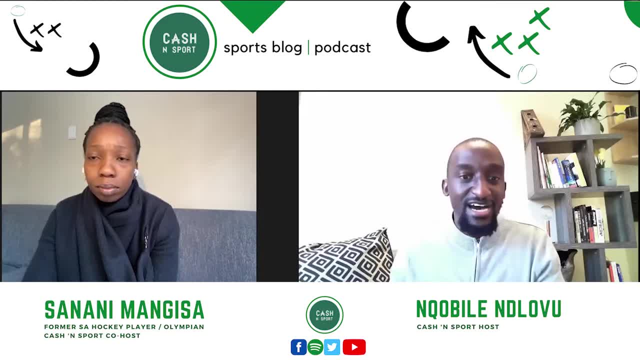 model of of the ioc itself. um, the ioc is a as an well, it's a privately funded organization, right? um, so let's take a look at it. where does the money actually come from? yeah, so so just to just to start off with, i absolutely love this. 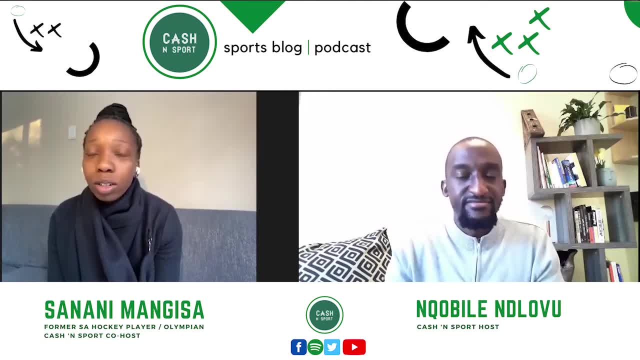 topic and the money around the olympics is really going to fundamentally change within the next few years. and i say that because we've seen the ncaa, you know, say that the athletes can earn money for their likability, their marketability, and and we're going to see that in the next few years. so 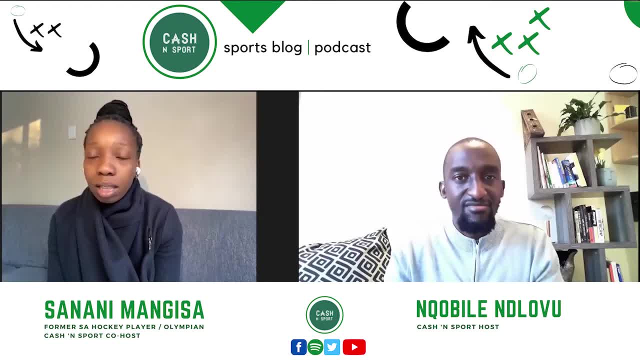 we're moving towards a, a time that athletes are going to be like: hang on, we're making you money and yeah, what's our cut in this? yes, money does flow back to the athlete through their nocs and stuff, and we'll chat about that just now, but this is really going to be in common interesting topics. 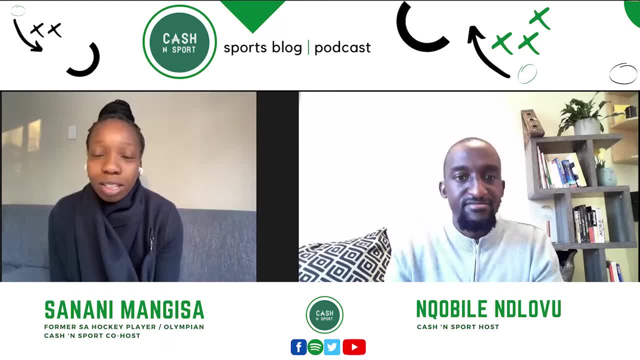 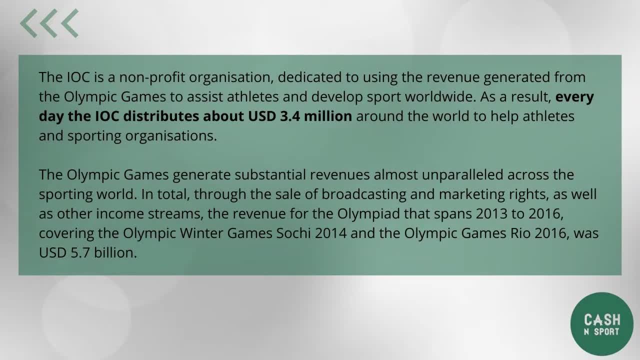 as the years go on, and and what i've always found interesting- and i'll now read it word for word- is that the ioc is a non-profit organization dedicated to using the revenue generated from the olympic games to assist athletes and development of sport worldwide. as a result, every day, the IOC distributes 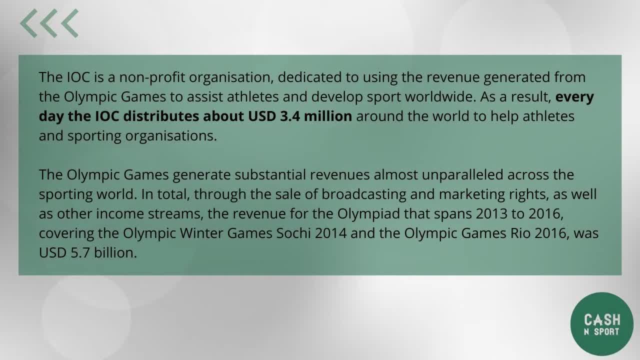 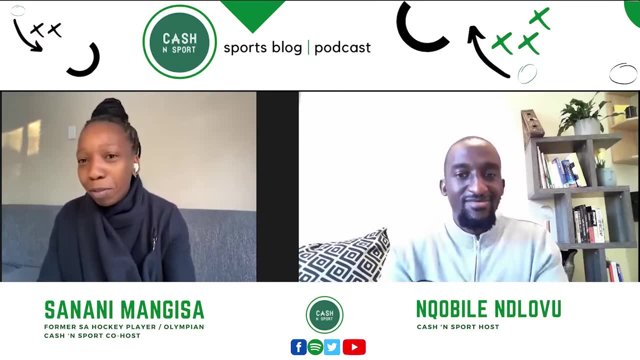 about 3.4 million US dollars around the world to help the athletes and sports organization. now, yeah, is the IOC really a non-profit organization on paper, on paper, but that's, that's a story for another day. but let's, yeah, let's look at the, the funding model of the IOC. 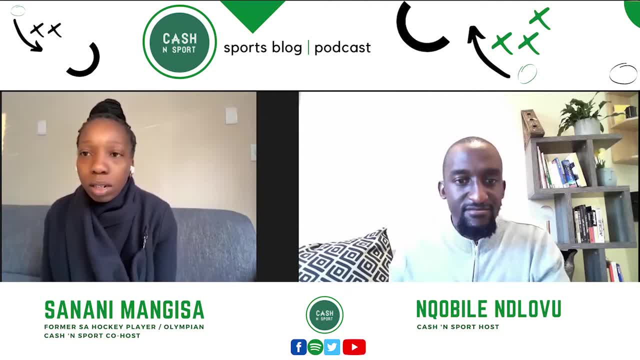 so the IOC. IOC is privately funded, so they get a pool of money from different sponsors and within the IOC you get your top tier sponsors. these are guys that sponsor the IOC specifically, so summer and winter games fall into that, and these are the guys that provide long-term 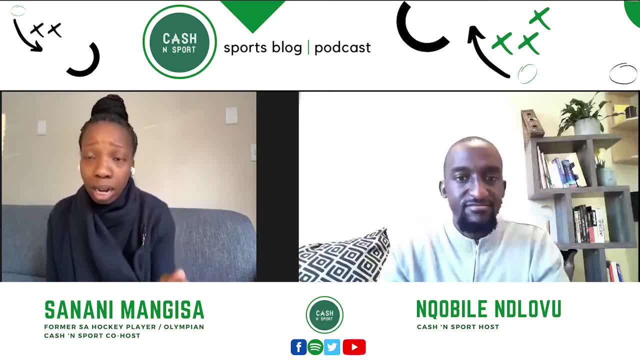 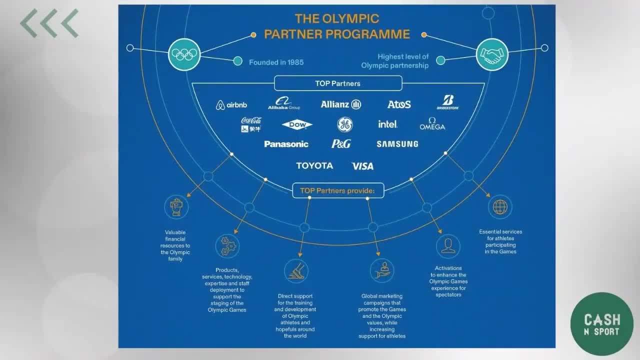 sponsorships of value in kind and also of of money, of money, cash, yeah. so let's just take a look at some of those sponsors. we've got likes of Alibaba, big Chinese e-commerce. you've got the likes of Bridgestone, the likes of uh Coca-Cola, uh Dow, General Electric, uh Procter and Gamble, HR's, the. 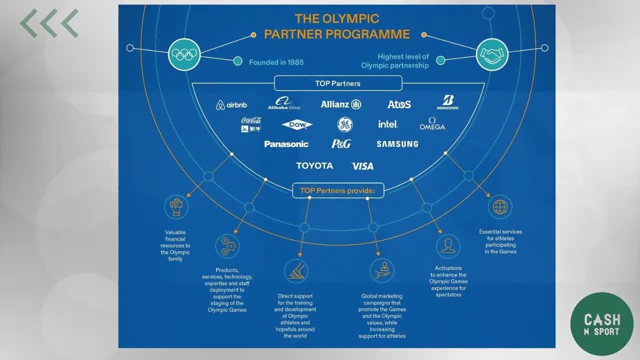 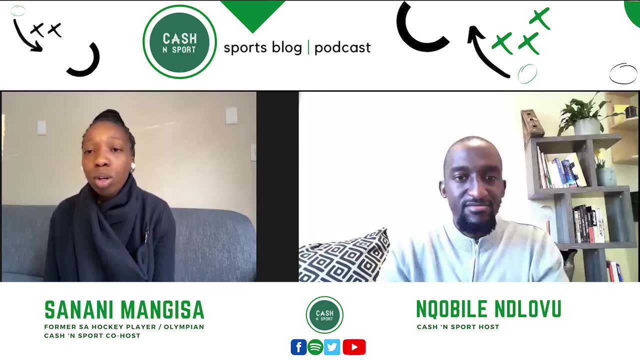 French, um, French IT company. yeah you, you've got a whole list of companies providing funds to the IOC, and I mean the longest standing one there, you know, household name Coca-Cola. so all these sponsors covered variety of things. they support the IOC in terms of all year round. um, they've. 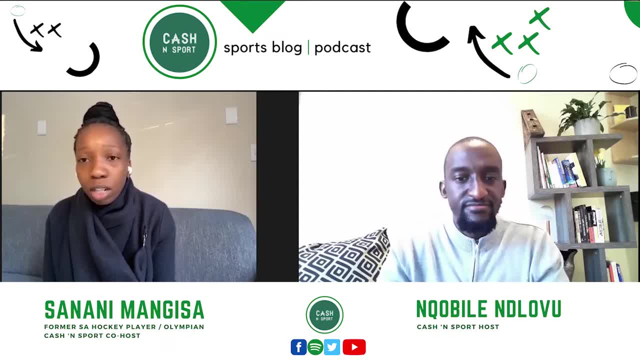 supported a variety of things and they, as I say, they give cash and they also give value in kind, which is where a lot of the the additional money comes from, or the additional value comes from, yeah, so yeah, that's that's uh. Olympic funding money that comes predominantly from from sponsors. yeah, and then we look at the broadcast of it- broadcast. 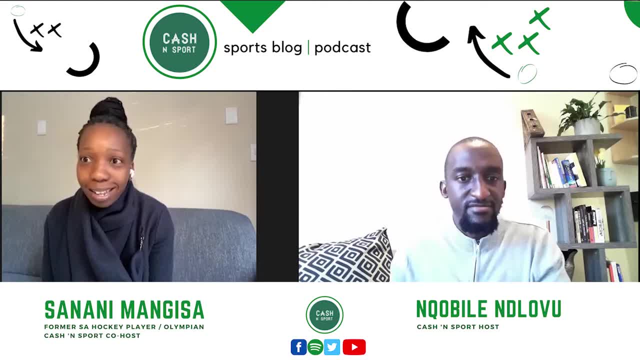 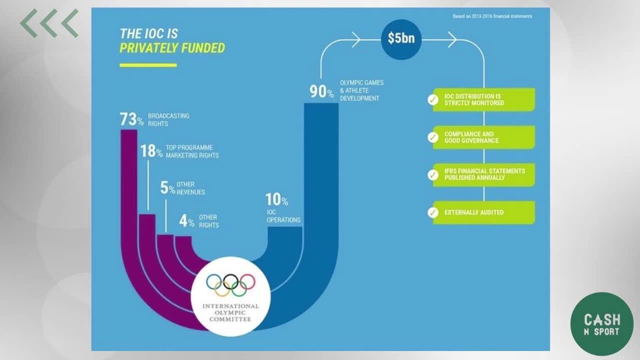 rights and around the IOC. a lot of money, yeah, a lot of money, and I think we we see it because you know, uh fans want to watch the Olympics. so what do broadcasters do? they go buyouts. they go buy the Olympic Olympic Games from the IOC, and that's where a lot of money is. 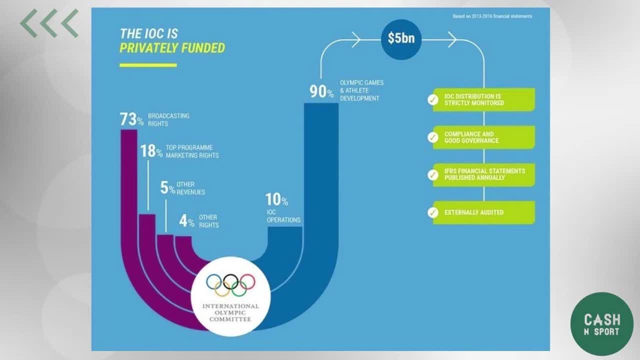 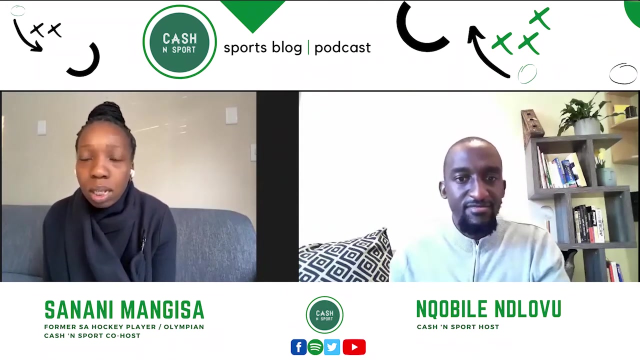 is generated. yeah, so we've got, yeah, so we've got broadcast, we've got the partners, we we've got also that other local organizing um sponsors which is like this year in in Japan. yeah, Tokyo will have sponsors, yeah, and I think let's, let's dive a little bit into that, because, because, if 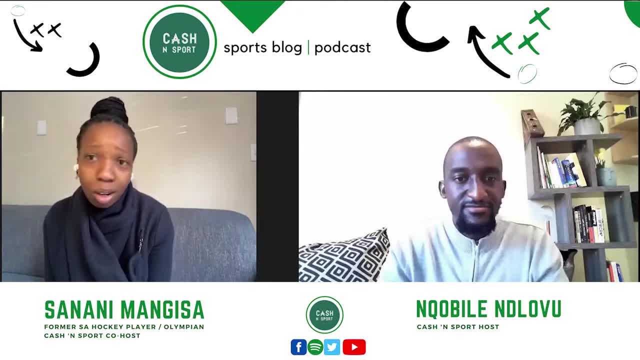 you are a beer sponsor in Tokyo this year, not a lot of people are drinking your beer because there's no, there's no big fan fairs, there's no big stadiums. yes, there are the big stadiums, but there's, you know, at 50% capacity. yeah, so with, with with these local sponsors, I mean more than 60 Japanese companies together. 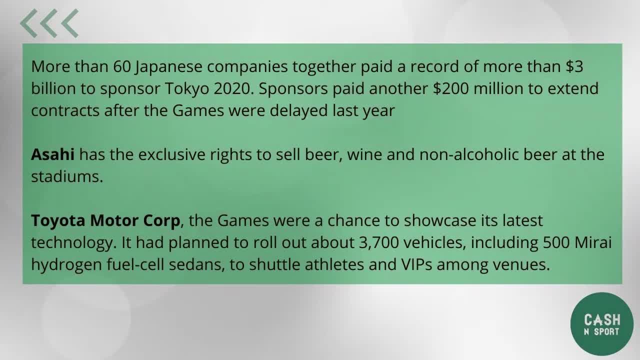 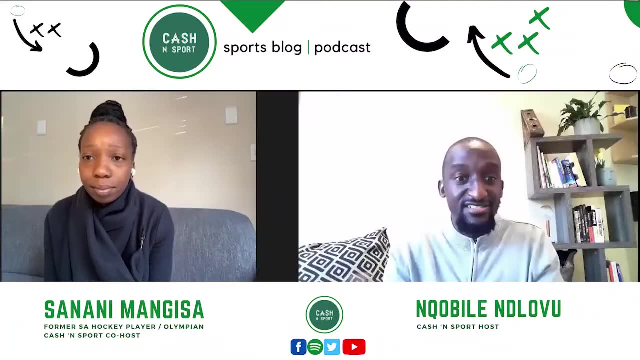 paid a record of more than uh three billion to sponsor uh Tokyo 2020. it then got cancelled and then the sponsors had to pay another 200 million to extend their contracts after the games were delayed a year. so already they've paid well 3.2 billion with in terms of local sponsors alone. um, but as 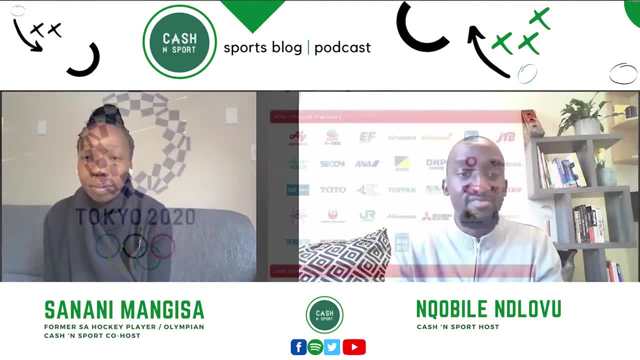 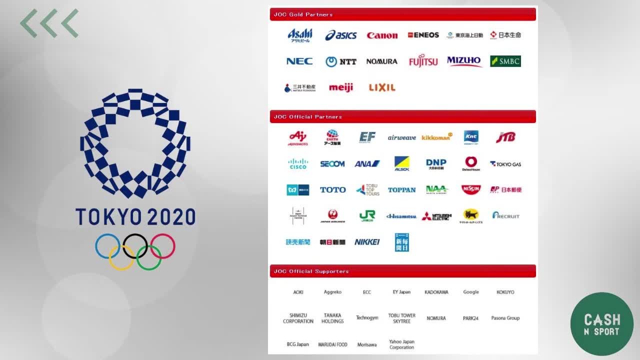 you say they're not going to get the full value because they're not going to be fans. for instance, Asahi, which is the official beer partner, was supposed to have rights to sell beer, wine and non-alcohol- uh, non-alcoholic, uh beer at the stadiums, but because it's not going to be fans. 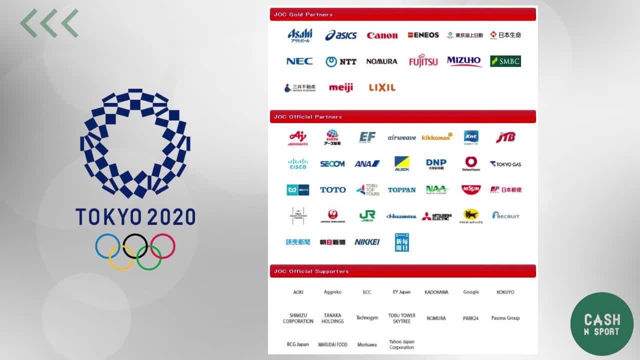 they can't do that. Toyota, which was the big Japanese um um motor manufacturer, was supposed to have the rights to shuttle vips and athletes to and from stadiums in their new cars, with this new technology, with electric vehicles and so on and so on. can't do that, and it's the same. they'll be able to do that because the athletes were still. 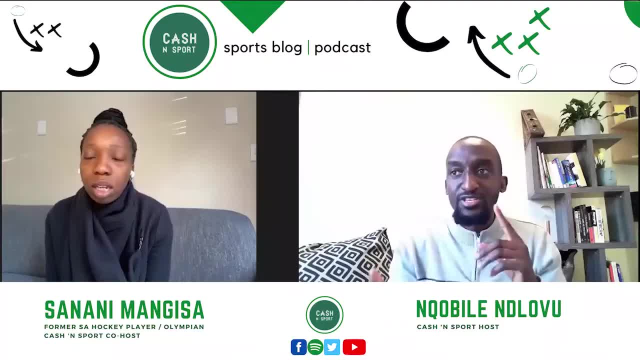 there, they'll do that. yeah, the athletes are still there, but but the larger group, which is which probably would have been much more important, would be the VIP's. so it's non-profit, but like the old things, like like the country old著, mm. I think there is a lot of refers in the industry, right. because in the summer of 2014, you know you get rid of the lights. the fans are going to have their athletes. I saw on the media it looks like people got stressed and going around taking pictures like they're not always taking, looking at theounding because the athletes are still there. I was. 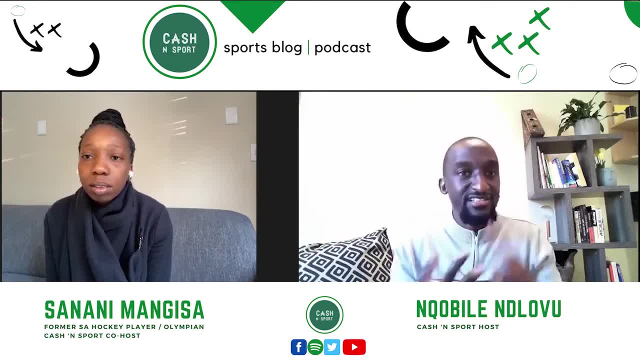 really shocked when I see them like the Hitachi inеныh trying to catch them. but you know, much more important would be the vips, uh, the guys who really have the money to to to make these purchases and and so on and so on, not going to be there. they've, they've rolled out the ads which 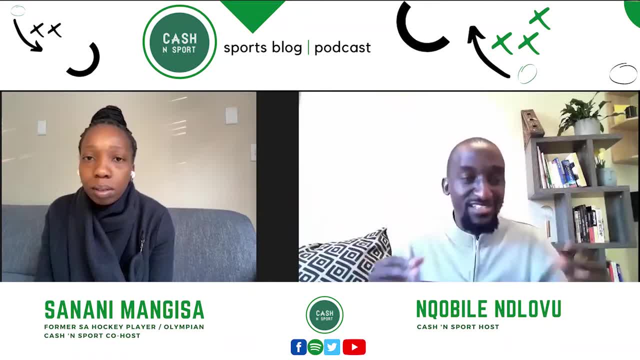 we've all seen the the toyota ads with this new thing, that, this new car that talks to you, etc. etc. but you know it's, it's just not, as it won't be as impactful as if if you had thousands and thousands of fans in the stadium. um, yeah, people attending. i think this is this, yeah, this is where it also 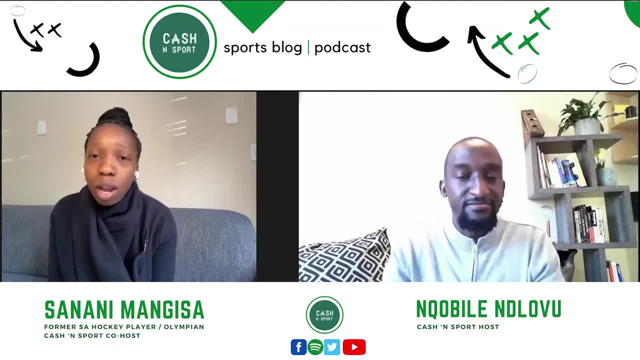 forces now sponsor to get clever on the digital side. so your ads, your digital execution, how do you touch the global audience that's not at in japan. so that's that's on marketing managers, marketing execs within these companies. now to say, okay, we paid for x and y rights and now they're. 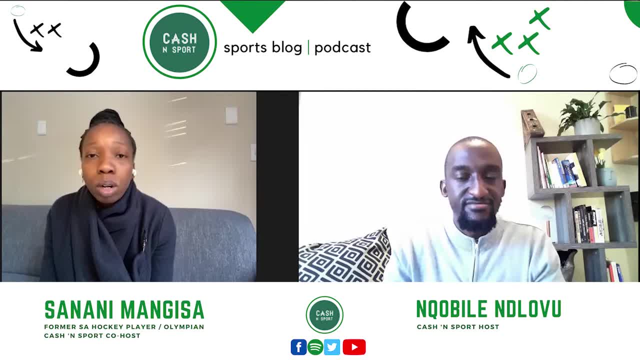 changing and that's apparently you know. reports are saying that's been one of um the top of meetings at the ioc to go. what additional rights can we give our sponsors in terms of the digital space? because no, you know, ioc has always held all their rights to the. 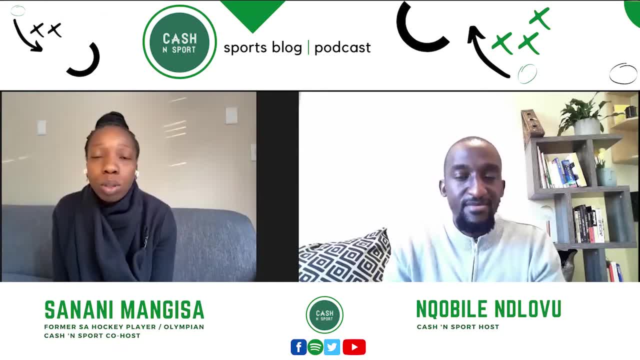 specific contracts quite tightly. but now, i'm sure this has to be a room of flexibility, but let's, let's just touch on the cost of, let's say now, tokyo, tokyo olympic games. yeah, they have ballooned to 15, projected at 15 billion billion. 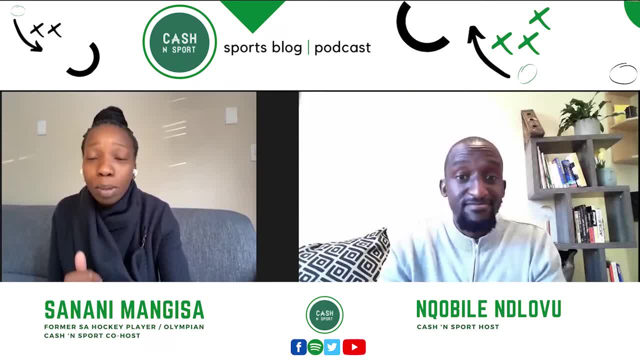 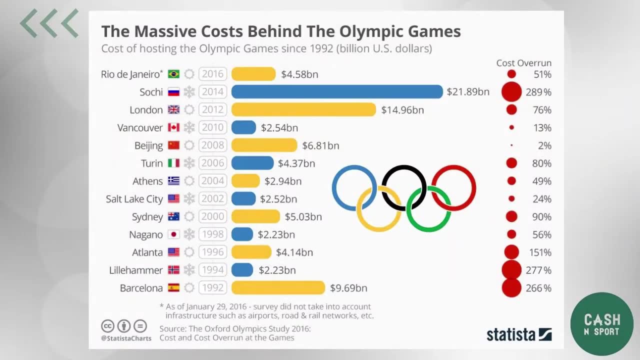 with the b, yeah, yeah, with a b: 15 billion us dollars, yeah, like, yeah, the. the costs of the costs are astronomical. i mean, if we look at the, the previous olympics, right, and just just to give people an idea of what the previous olympics have cost, uh, barcelona, uh, 92 cost 9.6 billion that. 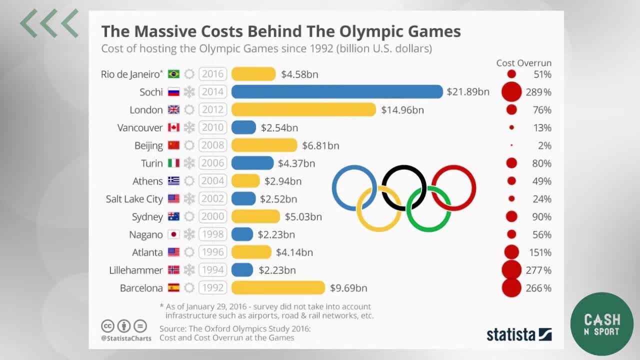 was the summer olympics: atlanta um 96, 4.1 billion. sydney, 5 billion. um athens in 2004, 2.9 billion. beijing, 6.8 billion. london was expensive, 14.6 billion, right, but you had the full benefit, fans everywhere, etc. etc. rio, much, much less. 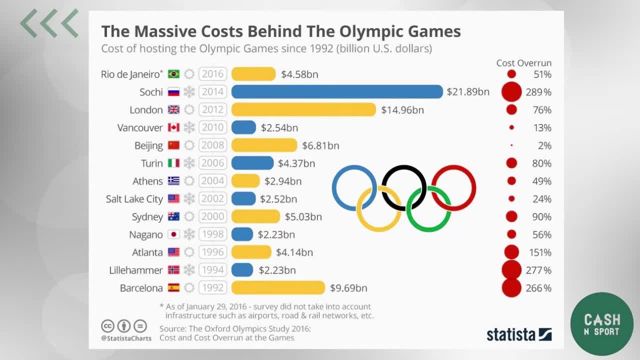 4.5 billion. now you're jumping up to 15. this is going to be the most expensive olympics ever. 15 billion dollars, 15 billion, that's an, that's an outstanding, that's. that's an outrageous amount of money, and and and. 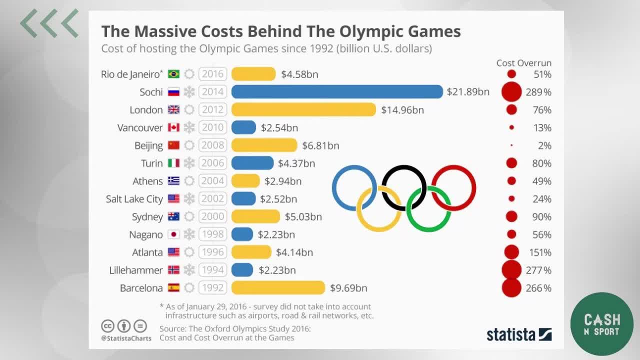 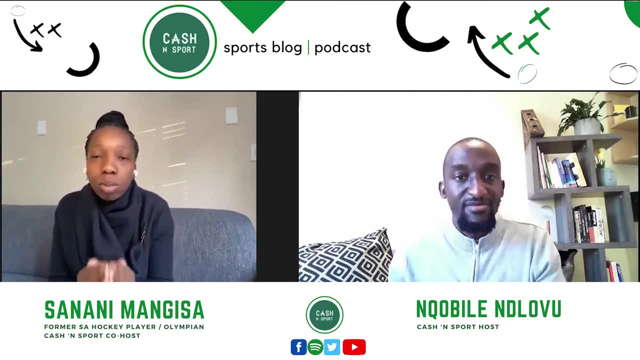 we get it like there's covert testing, there's bubbles, there's now. that's why the cost of balloon- yes, it's an additional year of everything- but the cost of bubbles around the covet 19 protocol. can this become sustainable? yeah, these, these costs are going to continue to escalate. 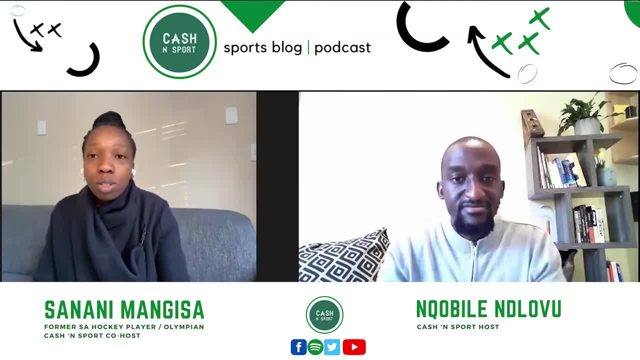 so, um, just a disclaimer: if you are listening to this on spotify, we implore you to watch the video of um, cash and sports. we have got a lot of diagrams and a lot, a lot of images that we've inserted just to show the projections of the money and the graphs. so, uh, nabs, one thing when we were discussing just now about 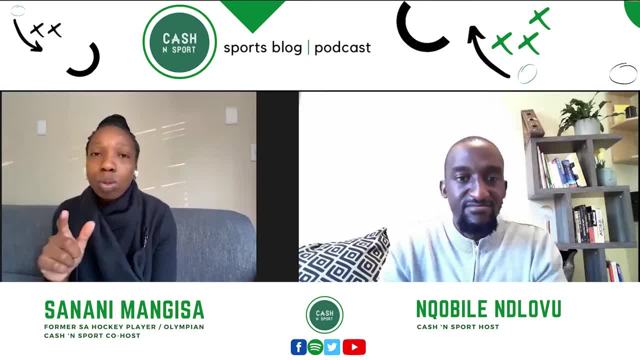 about the cost of the olympics is also the, the escalation of what was budgeted and projected to what the the games end up being. i think we also need to look at that. so because some games run 40 over uh, 50 percent over, um, i think the highest. 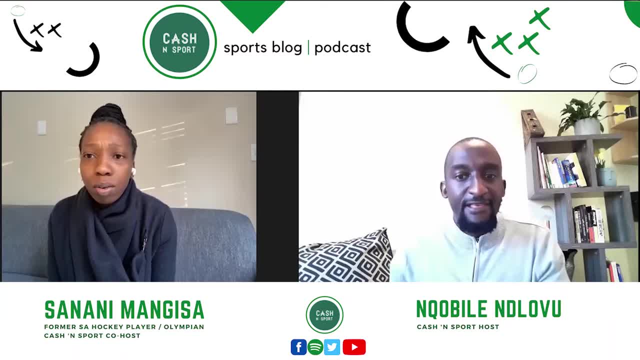 was uh, was it sochi winter, winter olympic games? that ran like 300 percent over? yeah, 289 percent, yeah, yeah, i mean even the, even the, the rio games were 50, 51 percent over. almost all of the games always run over budget. i mean london: 76 percent over, uh, van um, beijing was, beijing was almost. 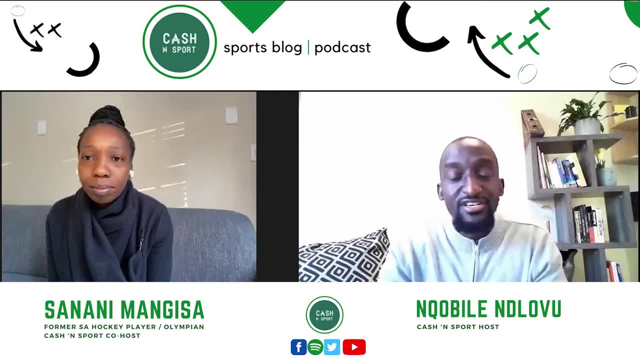 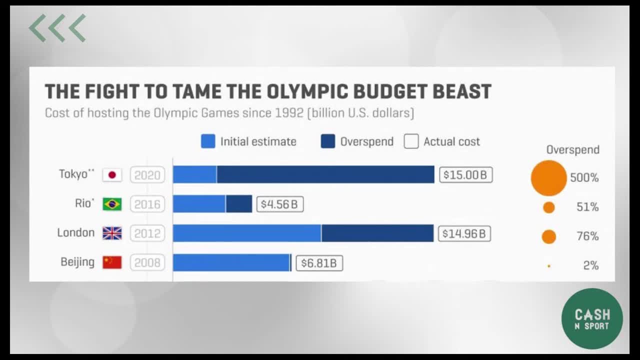 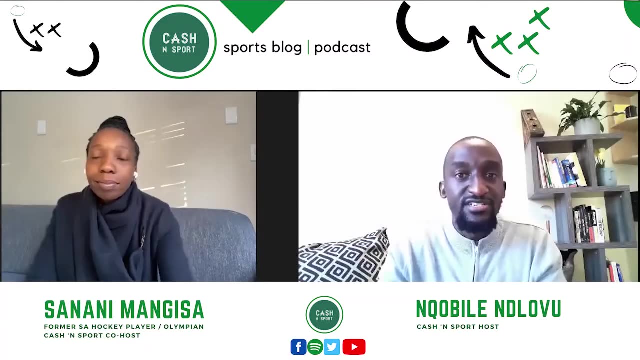 on budget just two percent over what they projected. so it's we, we've, we, yeah, it's we'll, we'll take a look and and give you guys the figure as well for what, uh, tokyo is predicted to be over by. but the the money is astronomical. it is, it really is astronomical. so 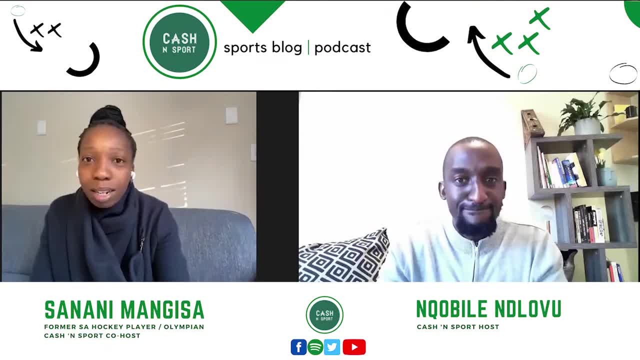 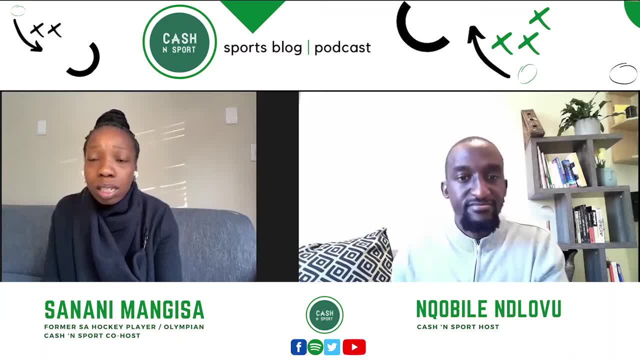 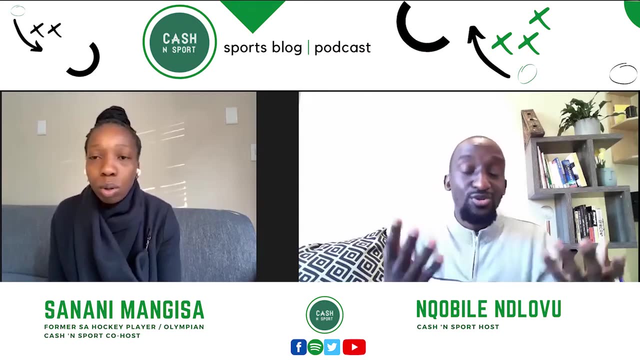 more. and and i think it's worth noting that um ioc hosts the games. you know you're hosted with the host city and then i see, move on to the next games. no, olympics pays off the the month they owe in that year. so i remember it was a couple of years ago. athens was in 2004. 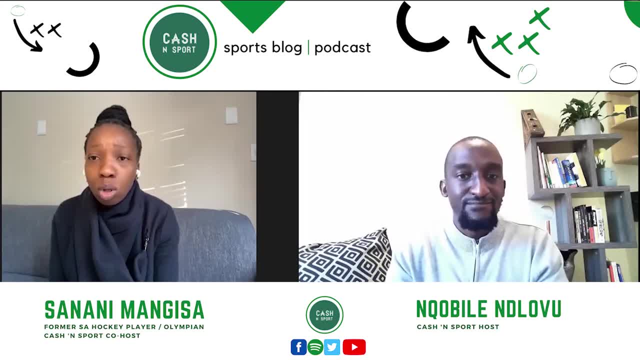 and i think it was only 10 years later that they fully closed off the books. that is huge burden to any host city. yeah, but if, if we look at it, if we ask the question: okay, so what does the ioc themselves? what? what do they contribute towards these budgets? you, you would be surprised if they. 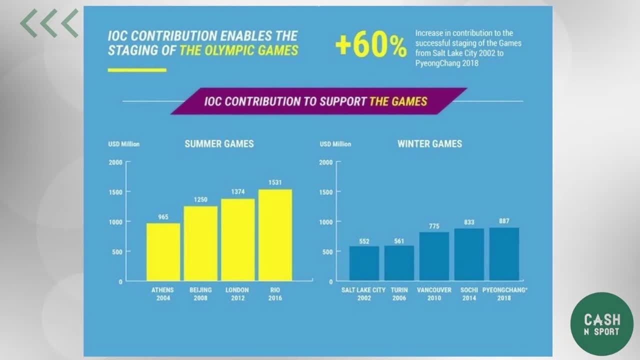 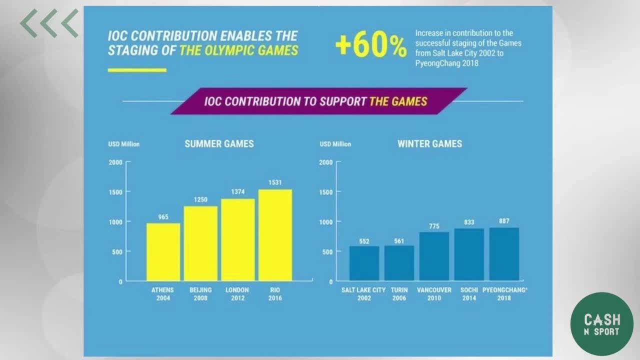 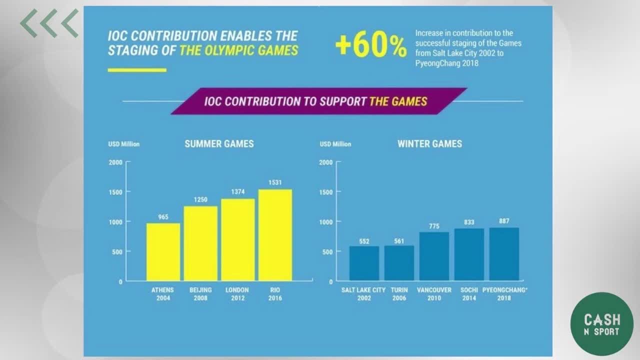 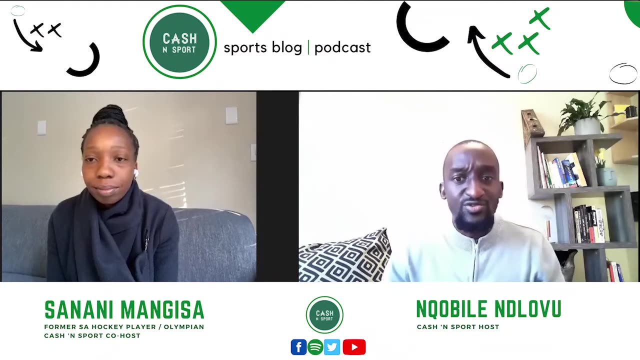 of the games themselves was a total of 4.58 billion. so they contribute, yeah, they contribute, just roughly what a third of the total cost. and then the local, the sponsors, contribute and the local organizing committee has to, has to fit basically the rest of the bill, the rest of the 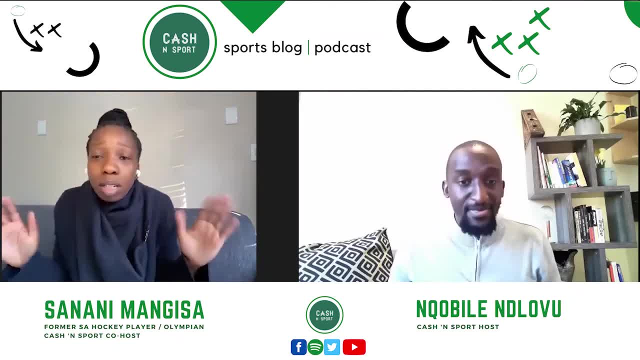 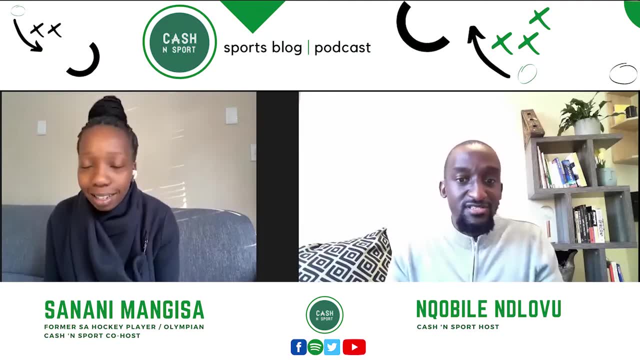 bill. yeah, this is why governments look at that amount and go, oh, we can't do that. you know, yeah, yeah, and it leaves you with a whole bunch of white elephants. you know, you exactly leaves you with a bunch of white elephants. look at rio: um, you know their stadiums are languishing. they. 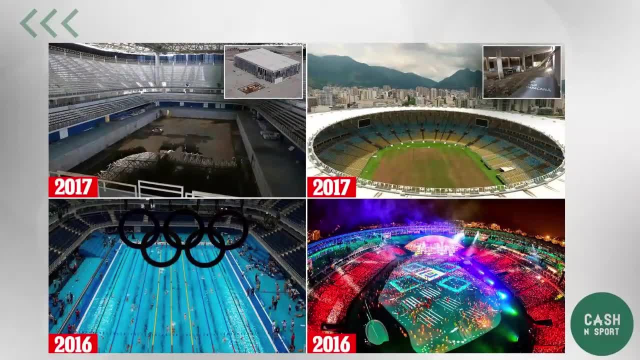 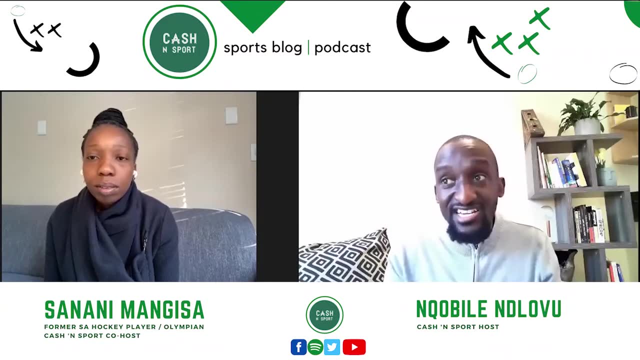 don't know what to do with them. it's the same thing with athens. you know it's, it's. does it actually work? does the model actually work and is it worth actually saying? this thing is a global event, spread it out amongst um, a number of cities hosting different. 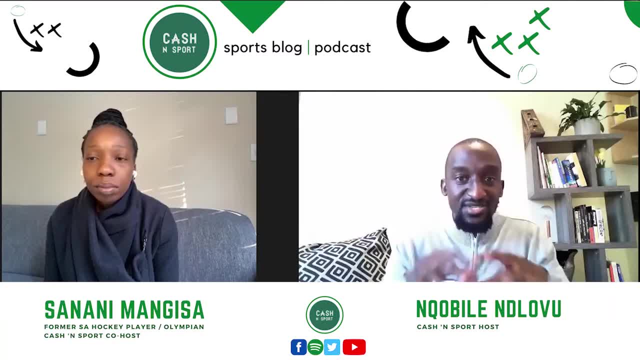 events and different cities at the same time and spread the load and allow more people to be- to be- um, you know- involved, or more countries to be involved at a cheaper rate. you know, i mean even this. yeah, um, olympics, here they're trying to make it the most efficient, um, in terms of um, you know how. 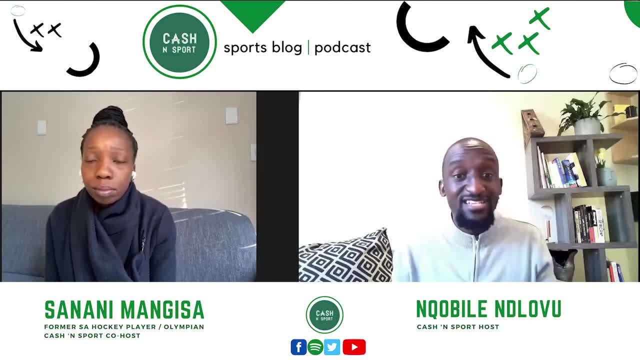 they, they run the games, but still 15 billion is 15 billion. you can't get away from that number. you know now, and- and this is this also comes into question- when you all come to play, when you question: why hasn't africa had an olympic games? come on, guys like 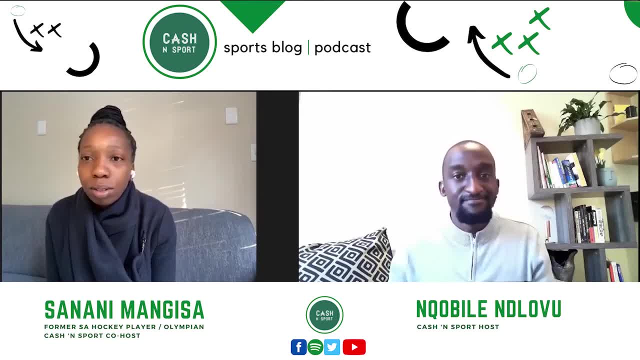 which african country has got 15 billion years exactly right now? and and also with our problems. i always go. i'm an olympian, i would love to have olympics in africa, but with the problems facing africa right now, yeah, i don't know. like even even commonwealth games, which is on a smaller scale. 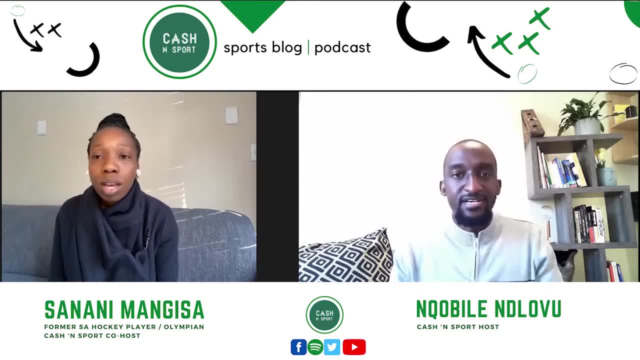 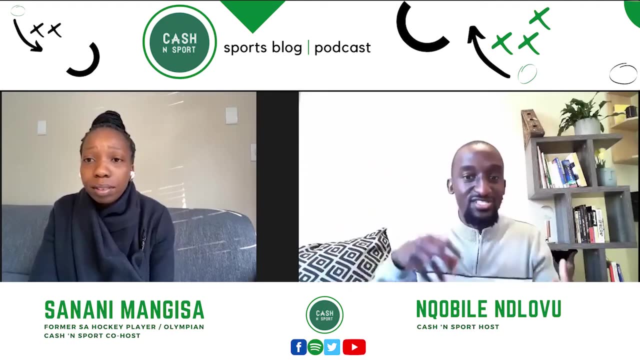 i'm going- it's just such a financial burden- to that hostage, to that government. it would be great, though, if, yeah, it would be great though, imagine if, if, if- we have one africa olympics, um, with with different events taking place across the continent, logistically it would be a bit of a. 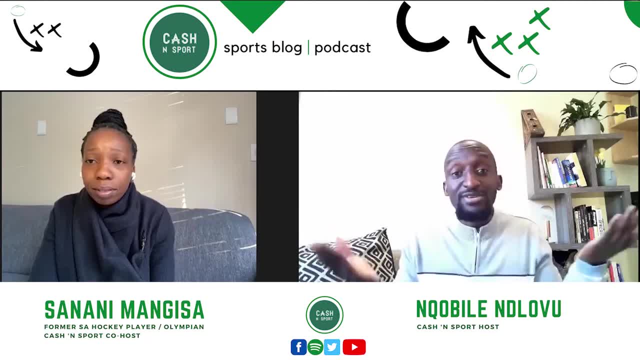 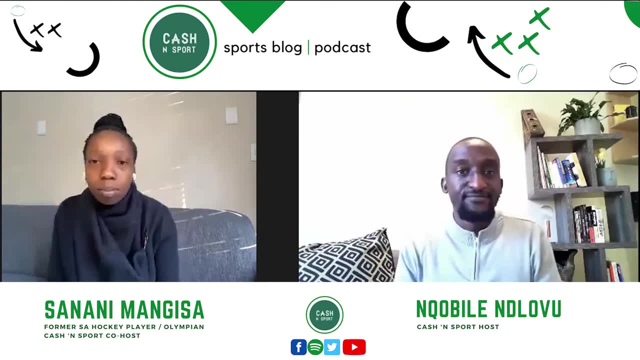 nightmare to try and put that together, but it would be cheaper and it would make probably more sense. but look, if you, if you know that your athletics, you in egypt, um, you know spread. or athletics in south africa, yeah, um, call it swimming in another country, you know, then, as 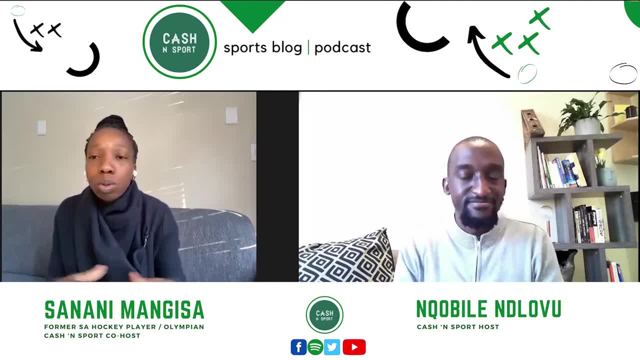 an athlete, you're based in that country. yes, yeah it. it dilutes you being one olympic movement, one, one, one, um. but it just spreads the cost. it really just spreads smaller olympic villages, um, yes, the branding around olympic village, those kind of things. it's small, but it's smaller villages. 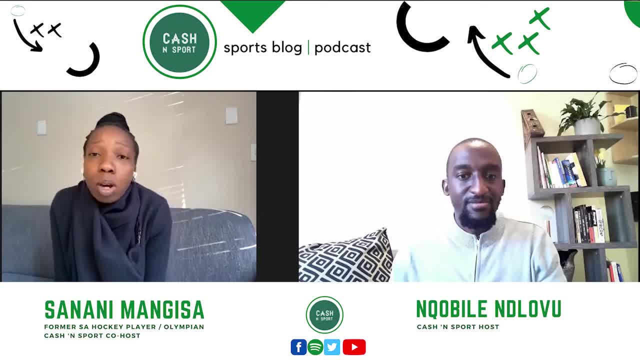 it's. it's less cost. no, it's an interesting model. i don't think we could write it off totally. it's an interesting model and something with maybe i see having a look at for the sustainability of the games, because that's going to come into question in the next couple of years. you're. 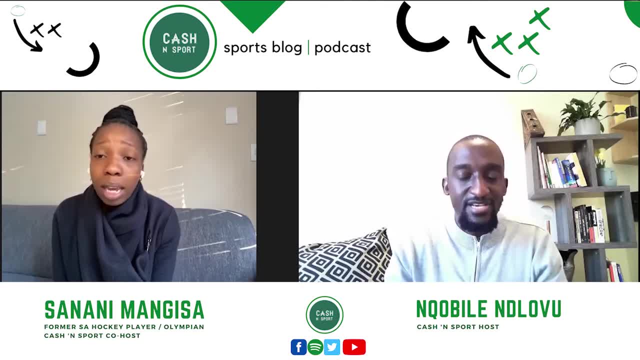 going to get a voice from the athletes going. we want to share the pie and also then we're going to get a voice from the host cities going. hang on, ioc. you guys need to help us more with the sustainability models, and they are there. there's there's definitely plans, future plans, uh, for ioc. 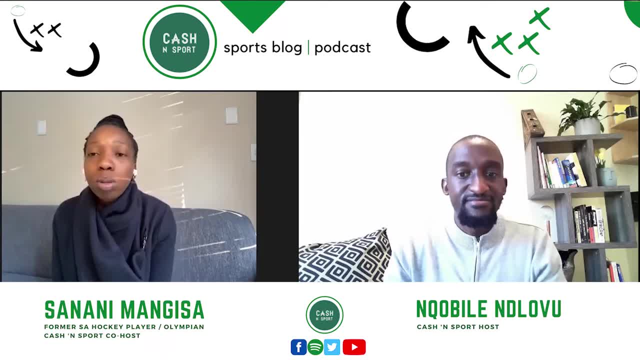 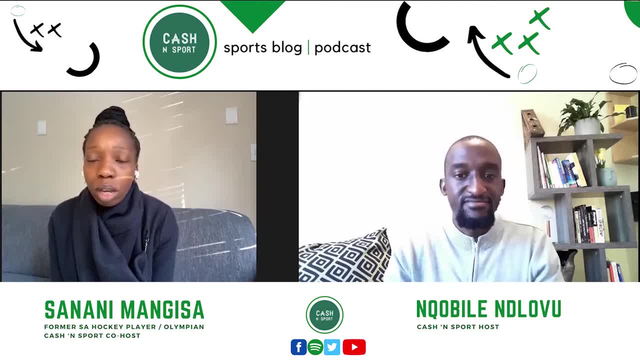 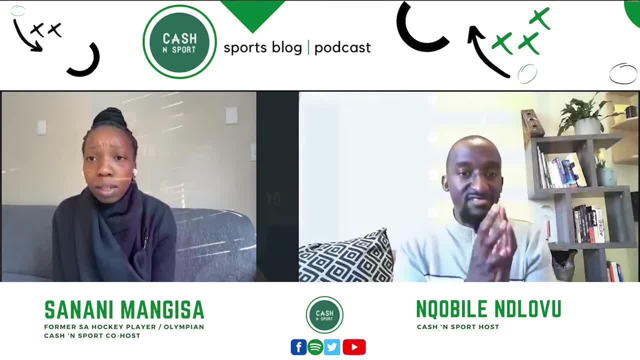 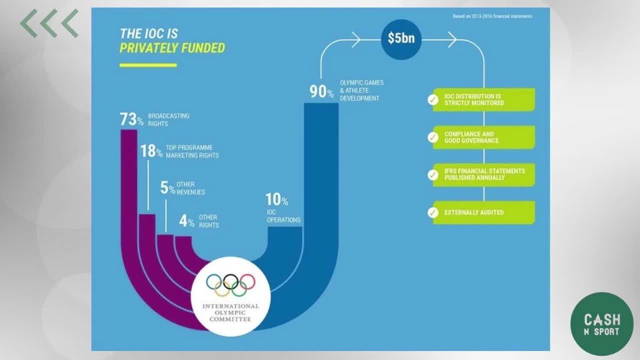 it's a problem of a recap right. so the ioc is privately funded, right. 73 of the money that that they receive comes from broadcast rights, 18 from the um olympic uh partners or sponsors program, which is toyota and all of those companies that we mentioned. um five percent comes from other. 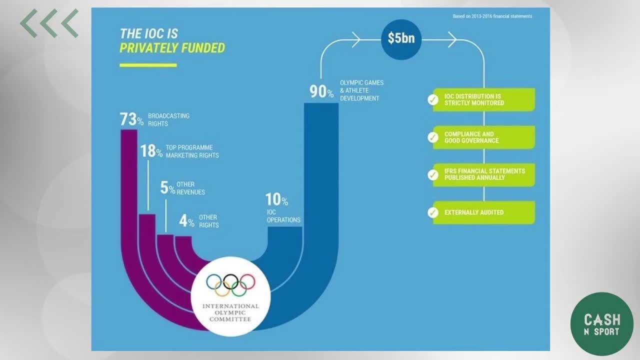 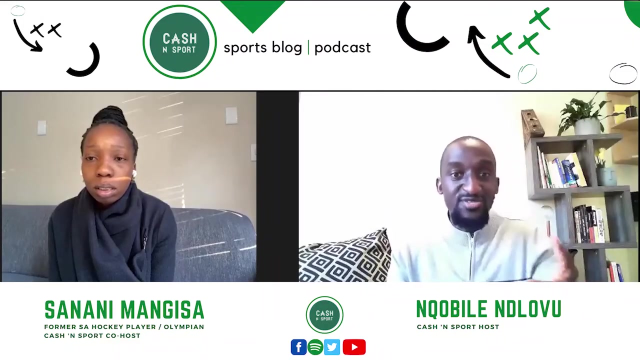 revenues and four percent from other rights. that money is then used in this way. ninety percent of it goes towards um, hosting the olympic games and athlete development. within that amount, zero goes towards paying well. remember we spoke about rule 40 a few weeks ago. rule 40 should kick in in about 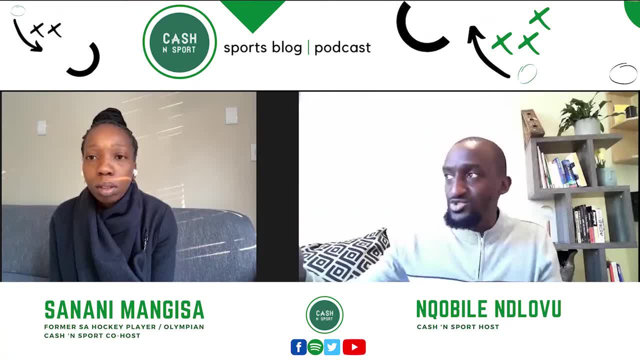 in about two days time, because i will be 14. what two weeks away? yeah, yeah, two weeks away from the olympics infiltration. it would be two weeks until the olympics comes out and where the athletes won't be able to earn anything, there will be no sponsors. sponsorship branding you, i mean, you were at the 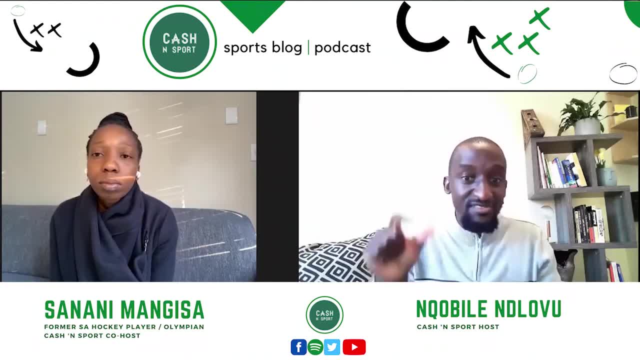 olympics, you can't wear your sponsor's kit, you can't, you know. so they're gonna have to figure that out, going forward with the ncwa ruling and so on and so on. they're gonna have to figure out how some of that component, you know, even if it doesn't go to the athletes directly, but they allow. 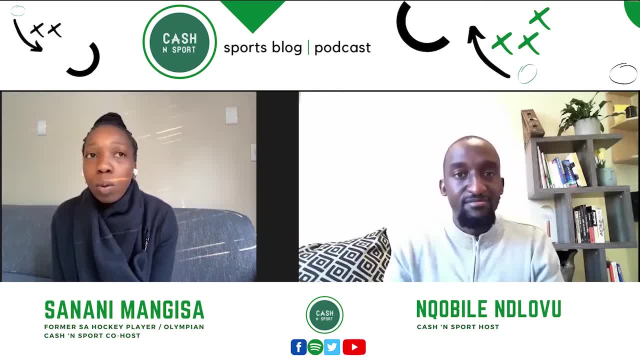 and- excuse me, don't worry- value for for what they're doing. yeah, but one thing we've got to emphasize is that some of the money also goes to the nocs- the local in each country, so the national olympic committee- and some of it goes to the federations of the different sports. so there's, there's money in that regard, but 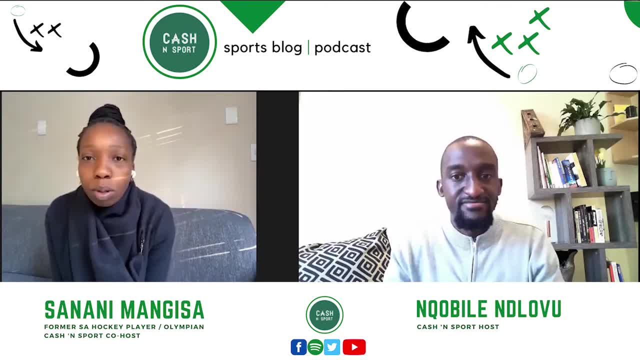 i think where it's going to come into play is. should, you know, be? should the olympics be a meet with cash prize attached to it, like the us open, like yeah, like uh, you know the, the relay games around the world, anything? should it be a money or should we keep it non-profit earning? 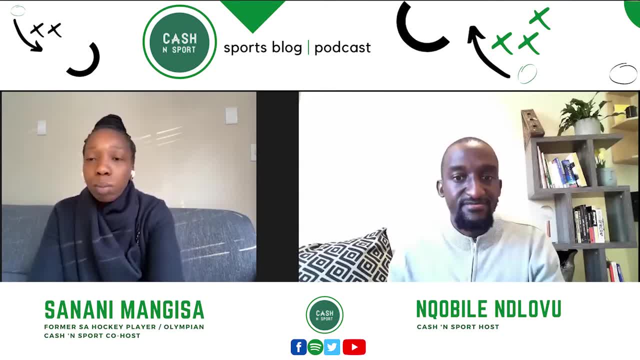 so these are the kind of questions that will definitely come into play, because athletes understand that they make bodies. they make, uh, yeah, broadcasters. they make. yeah, they are the product. yeah, they definitely are the product, and we're seeing the athlete voice become louder and louder, and rightly so. so let's watch the space, i guess. yeah, it's it, it can only become. 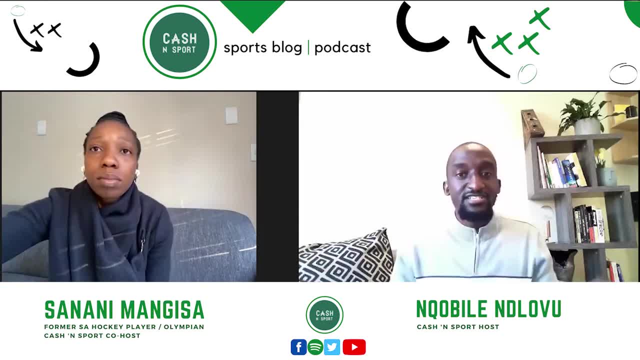 a a much bigger conversation, um, but let's let's take a look at one last thing before, before we wrap this conversation up: um, the money that they get from broadcasting rights, um, or the, the broadcasting fees that that are that are collected from from olympics, are massive. i mean, if we look 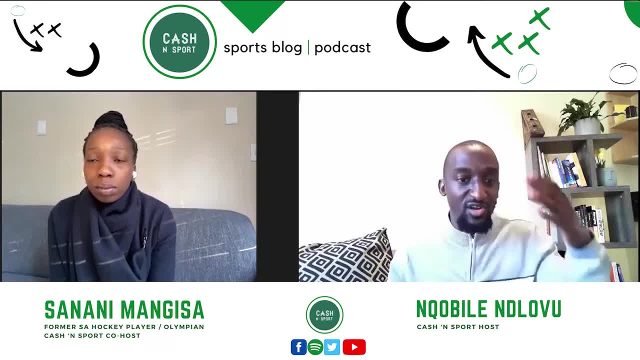 at just the number of people that are in the olympics. and the number of people that are in the olympics and the number of people who are watching in terms of the global audience is gigantic for an olympics um in 2012, the global audience was 3.6 billion people. um in 2016. 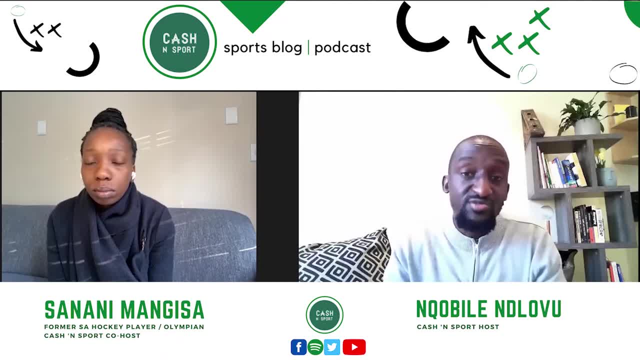 3.2 billion people this year. we assume it's going to be higher, because people are sitting at home. they don't have, you know, with with lockdowns and so on and so on, a lot more people are at home so they can watch the games. so we're assuming that we're going to get close to 4 billion people. 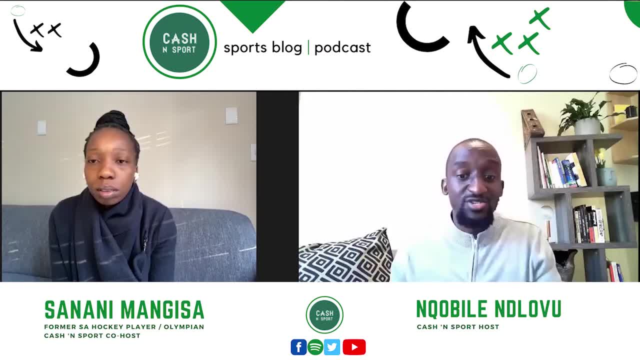 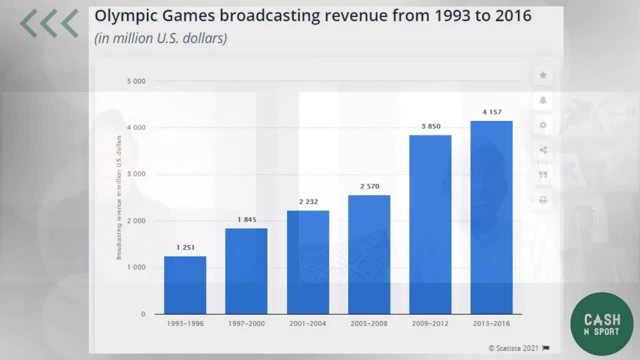 watching olympic games and the money behind it which these broadcasters pay is absolutely astronomical. i mean um in in 20, uh 20. between 2013 and 2016 there was 4.157 billion right that was received. um that was paid to the to the ioc from broadcast revenue. um in in between 2009. 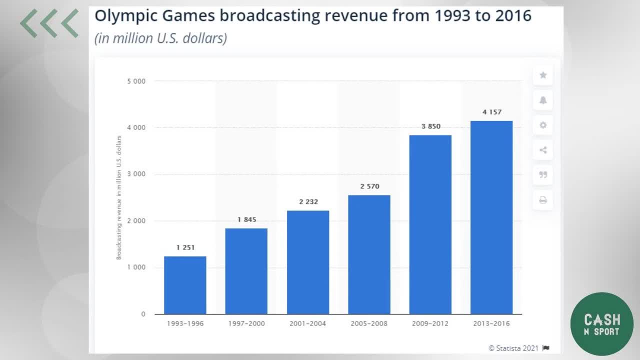 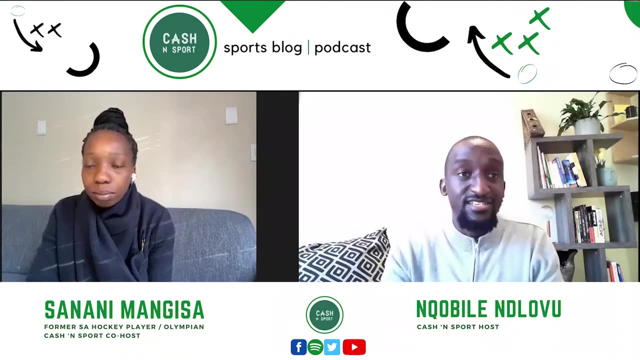 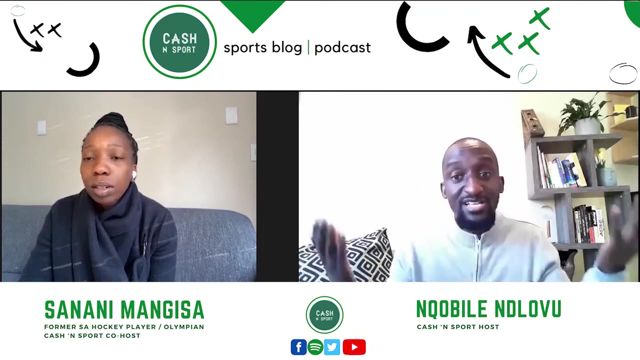 to 2012 it was 3.85. it's steadily increased, so it's heading towards four and a half, towards five billion. um, you know, and there's there's a number of different broadcasters. obviously they, they buy the rights and they put the, the content out, but they have to buy the right. super sport. 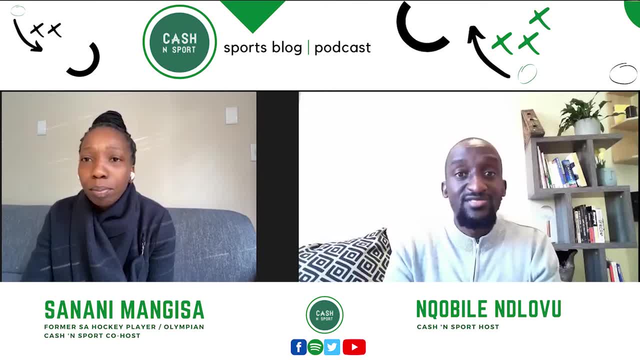 yeah, super sport and and the rest of them, and they buy the rights from the ioc. so the ioc completely benefits hugely, regardless of what's what's happened. yeah, yeah, so the ioc has done quite a nice model. they have what is called the olympics broadcasting services. 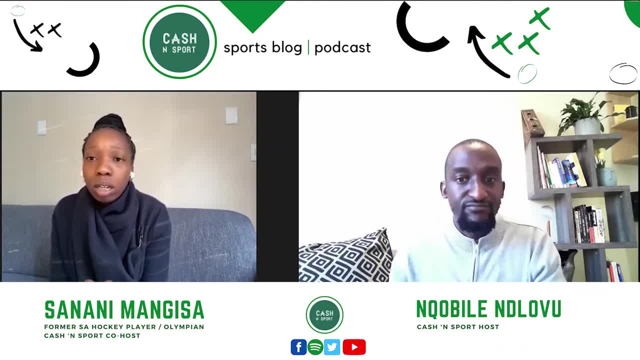 so these are the guys that are responsible for bringing uh the olympics to life on media, basically, yeah, so to protect everything of of rights around that space they're going, we'll do all the fees, all the media, we'll just syndicate it to the different broadcasters. so 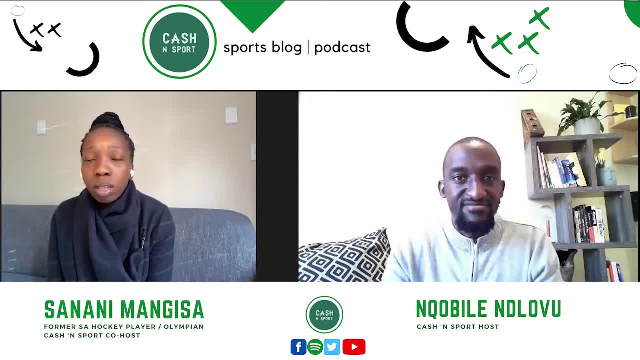 broadcasters really pay a lot of money. i mean, you've got the american guys, you know that pay a lot of money. uk, uh, you know different broadcasting houses in the uk. super sport is a big player there. smbc will buy the rights as well. um, you know, we'll have olympic rights, so a lot of the global reach. 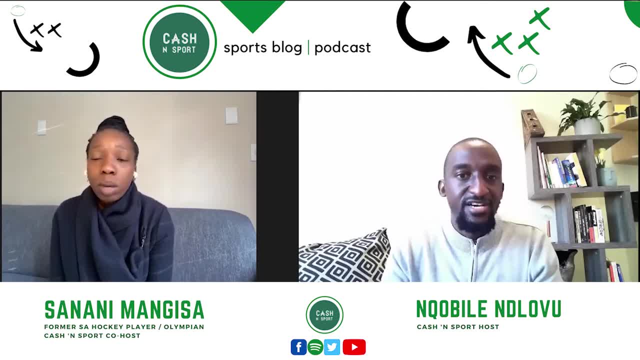 is quite big, and that's what ioc wants to do, basically is make sure they've got a wide- you know it's wide and it's deep- um and and a bigger global reach. so, as we, as we say, the numbers are probably going to be high, um, but also high, but. 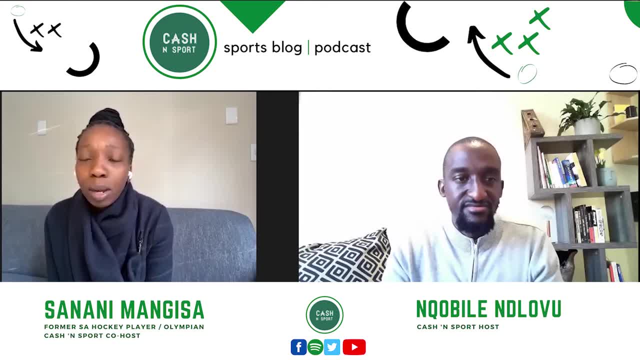 maybe shorter, because we know that you know attention spans of people and also the time difference comes into play with japan, so it will be interesting but that that is where the bulk of the ioc money is made from broadcast right and that's why you can understand why these guys are. 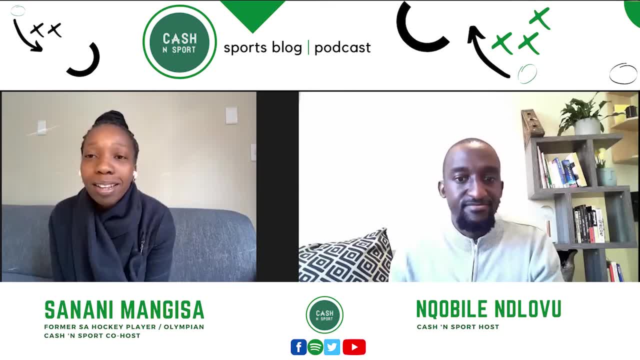 pushing on. you know, even without without, without fans in the stadium, they're going. no, uh, the you know, the model is that our games will go out live to billions of people, and that's what we'll. they're looking for that global reach. so even without fans, these, they'll still make money. 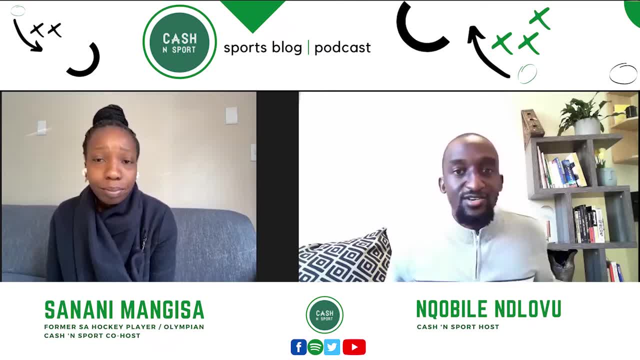 yeah, yeah, i, it's, it's. it's going to be an uh, a very interesting one to see what the fallout looks like and what france looks like in, uh, what is it? 2024? um, you know, there's, yeah, there's there's a lot going on in terms of discussions around um. just the funding, the, the, the way that sponsors 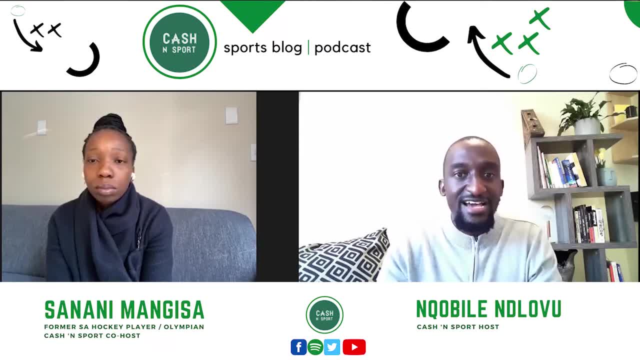 can act and act in a way that they can act in a way that they can act in a way that they can act, actually leverage off of their, off of their athletes and their assets. um, and just how this, this age-old tradition of the olympics, needs to change and come into the modern age, because 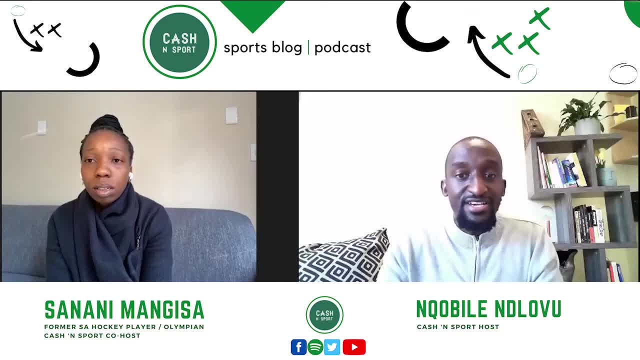 really it's. it's stuck a bit in the dark ages if you, if you look at it as a, as an institution and and in the way that they work, it's worked for them prior previously, but i don't see how it can it can continue to work in the long term. 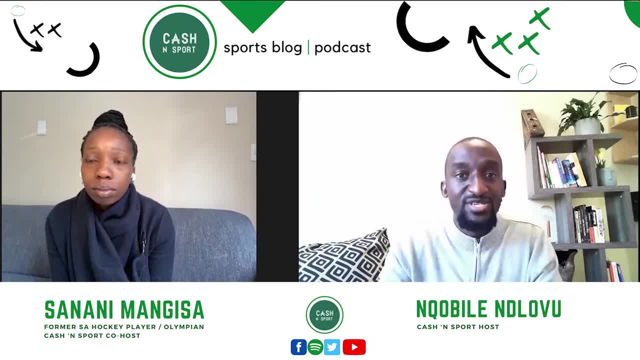 it can continue to work in the long term and cost um local organizing committees so much money. yeah, without them getting real value, um, you know, and and without the the athletes earning from it. you know that that ncaa ruling is so pivotal, and it will, it will, it will cascade down through the olympics, through. 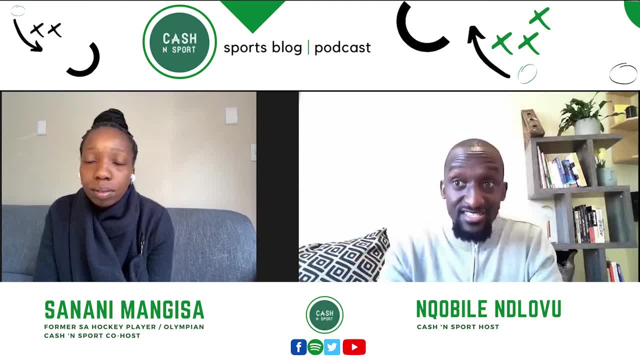 other sports in general, you know where you'll see kids earning big money from um, from from from their their careers, and rightfully so, as they should, because i mean athletes careers are short. you know, 35 years old, you're done. 30 years old, you're done so. 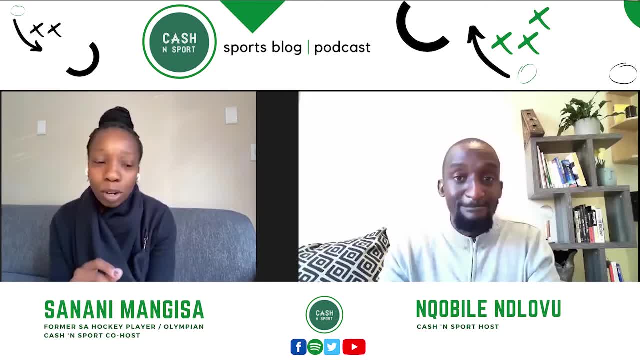 yeah, so just one last point on that is that, on on sponsors and money, i'm going to be very interested to see where all the merchandise goes. you know there's merchandise that was made for these olympics- yeah, one with 2020 on them, so the logo is staying the same, but there's a lot of. 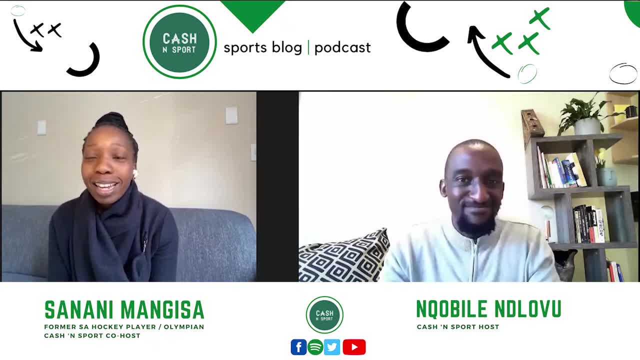 that's not changing. but there's this. all this ticketing and and licensing apparel merchandise caps this because the japanese locals can only buy so much of it. usually it was made for the international fans coming in. you'd buy a towel, you buy months, you buy this memorabilia. this is. 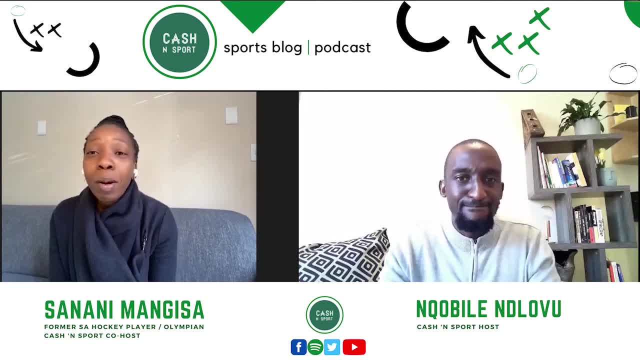 going to be a big black, dark hole in japan where all of the stuff has to go to because no one's going to buy nearly, yeah, anywhere near as much as would have been bought before, exactly. so that's a your big money money loss there. yeah, well, they, they have to figure it out, um, but at the end of the day, that's where we 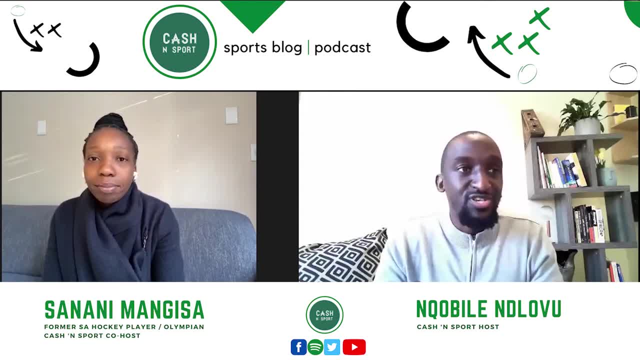 are 16 days away. um. you know we, we're going to start seeing a little bit more of um. you know of the action really really hotting up um qualification is basically done for for most, if not all of the athletes, for all sports um and we, we're we're here um squads are announced. 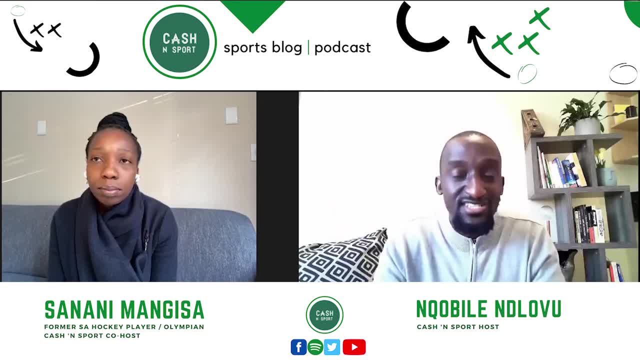 um and yeah, we're here. we are for 16 days away, literally just over two weeks away from the beginning of the olympics. thank you so much for joining us, guys in episode 10 of olympics. talk with myself and sanani. um, smash the like button, follow us on twitter. um and yeah, check out the.